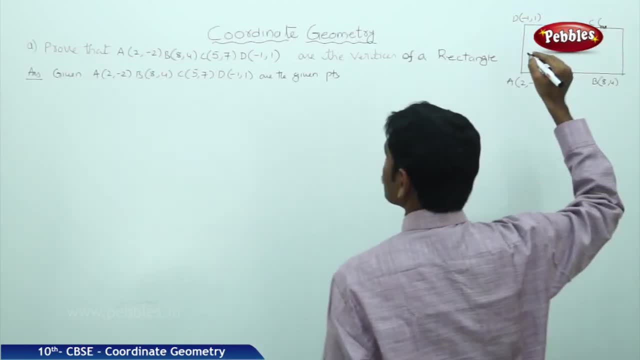 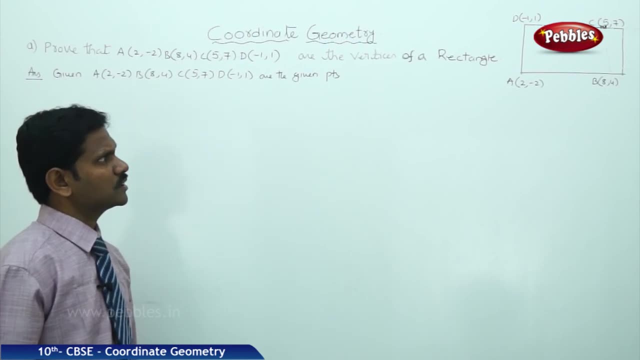 c of 5,7 and d of minus 1,1 are the vertices of a rectangle. Now we have to prove that these points are rectangle forms. a rectangle, First part: length of a, b, a of 2, minus 2, b of 8, 4, x1, y1, x2, y2.. 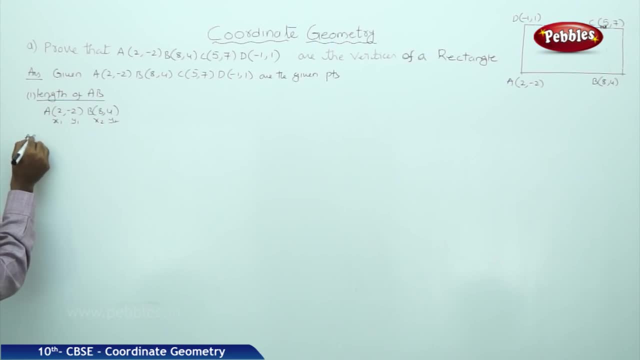 a. b is equal to root over x2 minus x1 whole square, plus y2 minus y1 whole square. That is a. b is equal to root over x2, 8 minus 2 whole square, y2, 4, y1 is minus 2.. 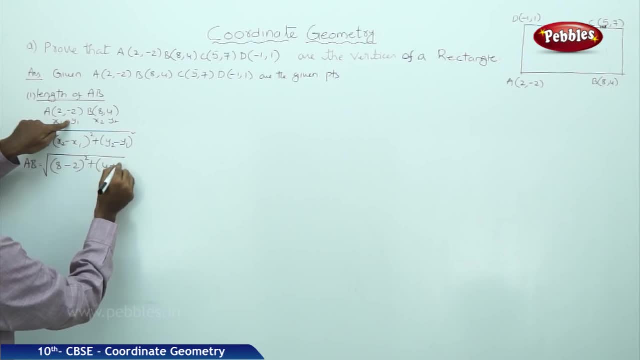 That is minus of minus plus 2. whole square, That is: a? b is equal to root over 6 square plus 4 plus 2, 6 square. a- b is equal to root 36 plus 36.. a- b is equal to root 36 plus 36.. 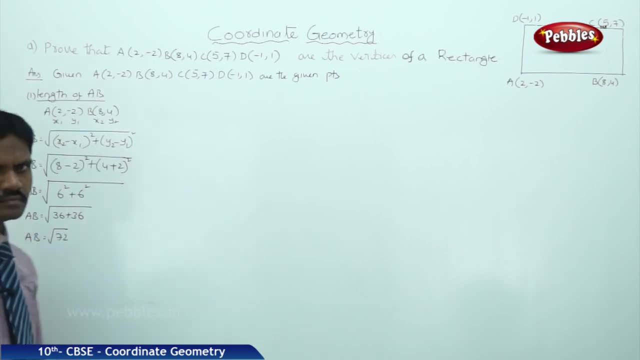 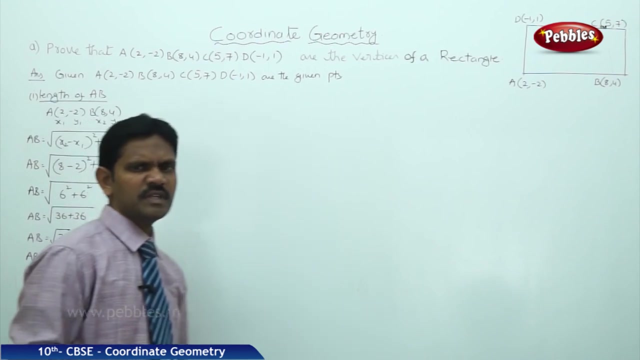 a. b is equal to root 72.. That is a- b is equal to root 72 can be 2 into 36.. That is equal to 6 root 2 units. That is a. b is equal to 6 root 2 units. 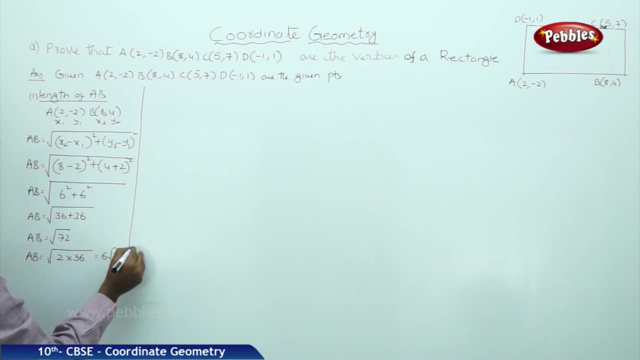 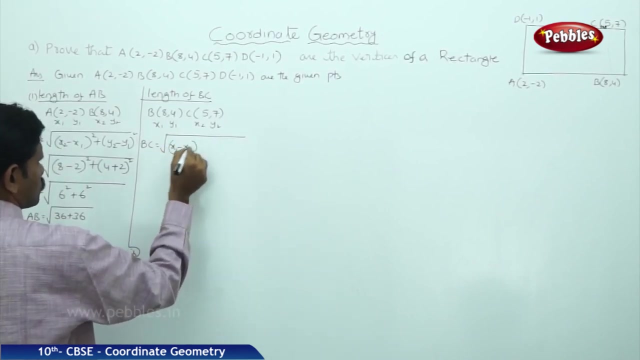 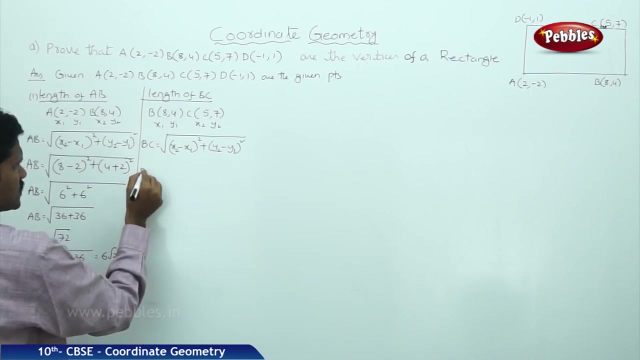 Now length of b c, length of b c, b of 8, 4, c of 5, 7.. That is x1, y1, x2, y2.. b c is equal to root over x2 minus x1 whole square plus y2 minus y1 whole square. That is a. b c is equal to root over x2, 5 minus x1, 8 whole square plus y2, 7 minus y1 whole square. 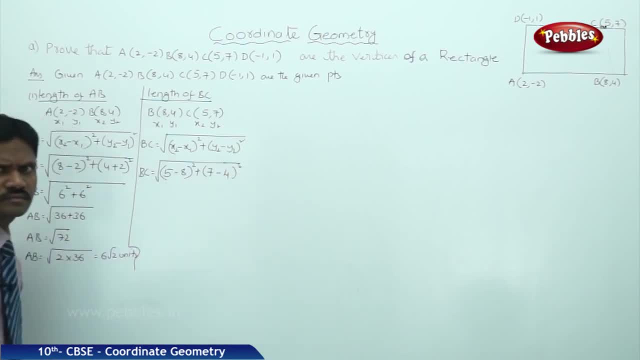 b c is equal to root over x2 minus x2 minus x2 whole square plus y2 whole square. b c is equal to root over x2 minus x2 whole square plus y2 whole square. b c is equal to root over x2 minus x2 whole square plus y2 whole square. 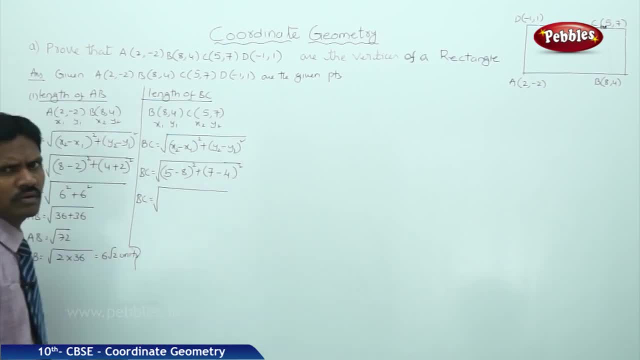 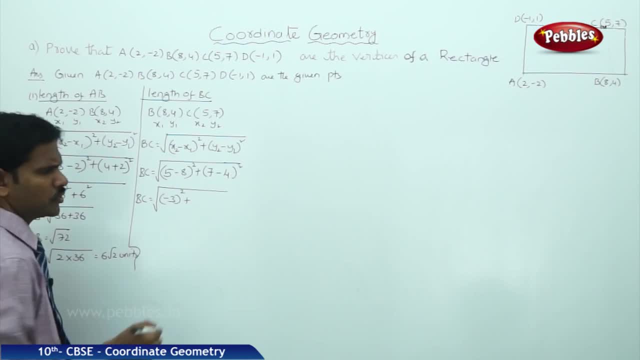 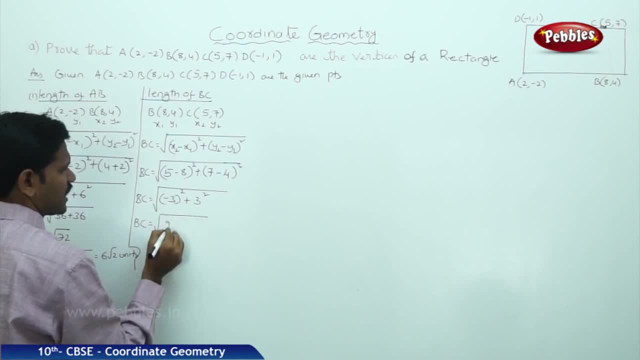 There is a BC is equal to root over 9 plus 9,. 9 plus 9 can be write as 2 into 9.. That is BC is equal to root. 9 can be break down into 3, 3 root 2 units. 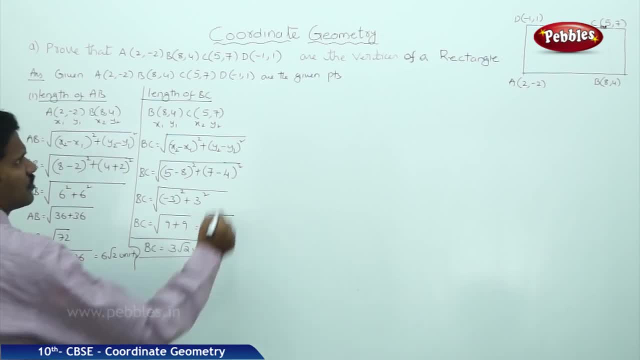 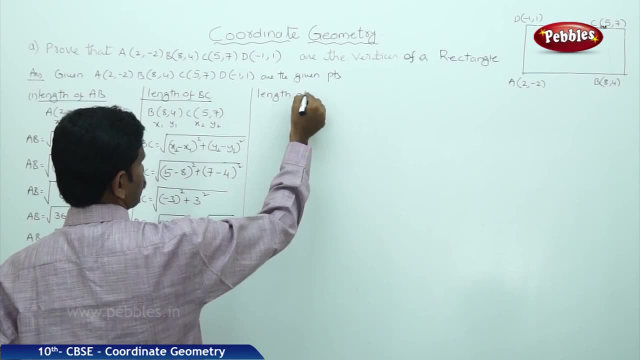 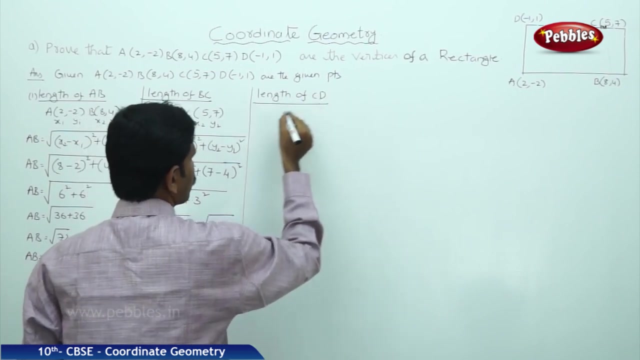 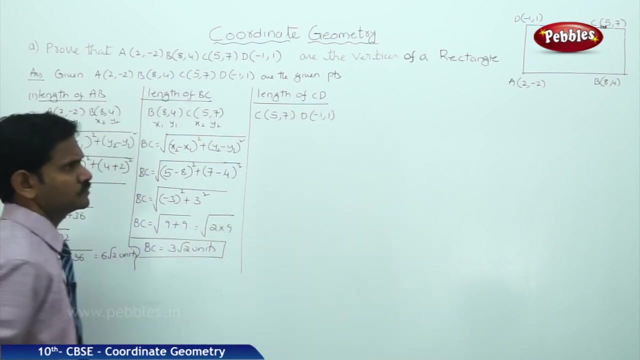 Now the length of the BC is equal to 3 root 2 units. Now length of now: AB: completed BC. completed. Next length of CD: C of 5 comma 7, D of minus 1 comma 1.. X, 1, Y, 1.. 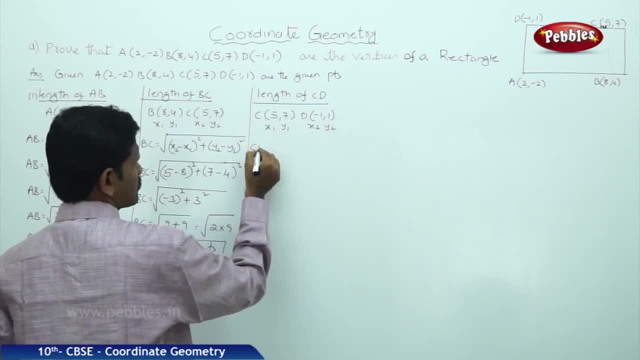 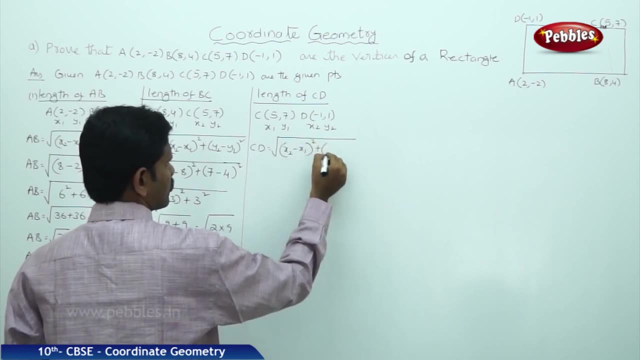 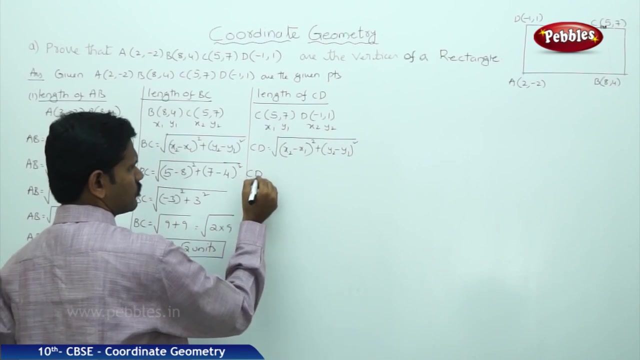 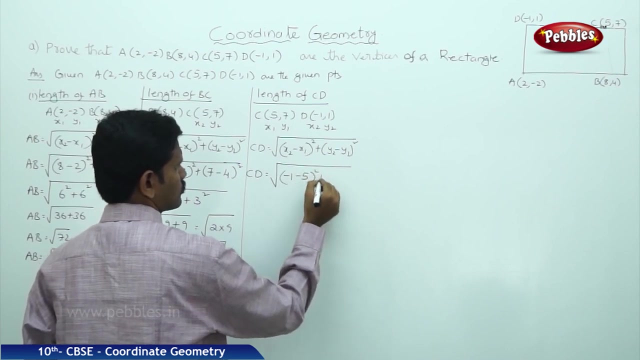 D of minus 1 comma 1.. X 2, Y 2,, that is CD, is equal to root over X 2 minus X 1 whole square, plus Y 2 minus Y 1 whole square, That is CD, is equal to root over minus 1, minus 5 whole square plus 1 minus 7 whole. 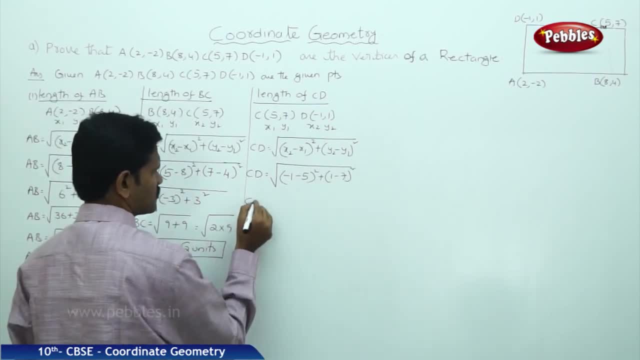 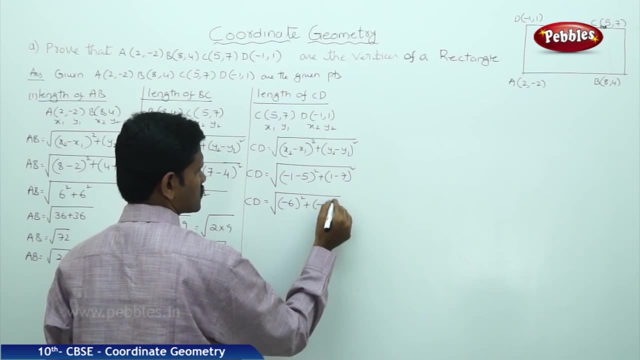 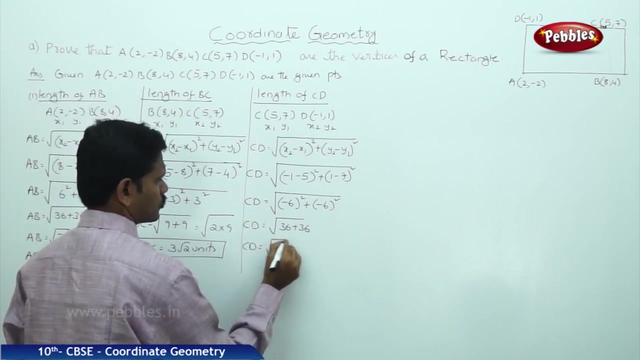 square- That is CD- is equal to root over minus 6 whole square. minus 6 whole square- That is CD- is equal to root over 36 plus 36.. CD is equal to root over 2 into 36 can- That is CD is equal to root. 36 can be written as 6, 6 root 2 units. 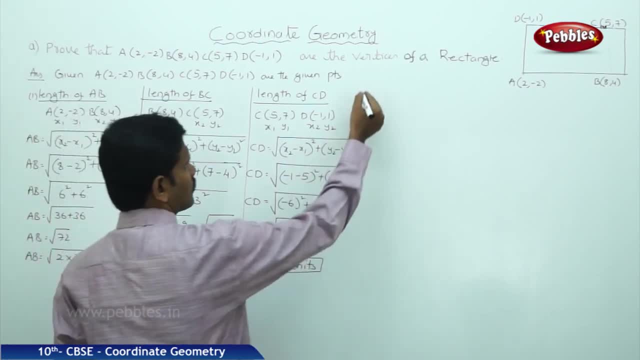 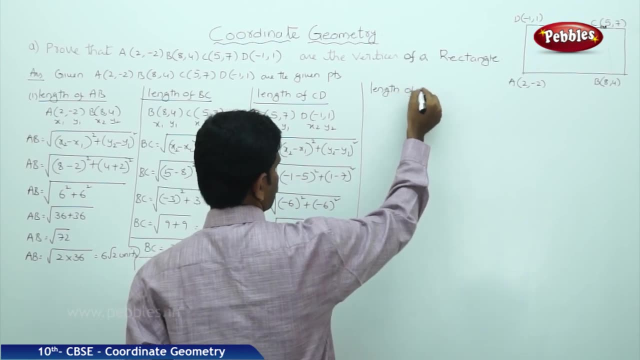 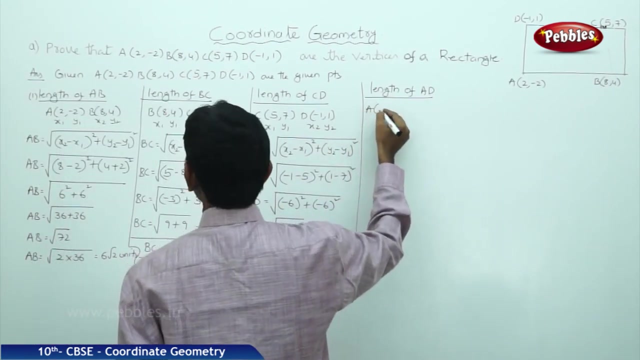 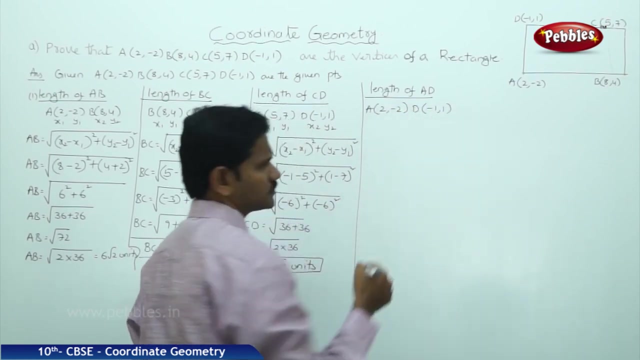 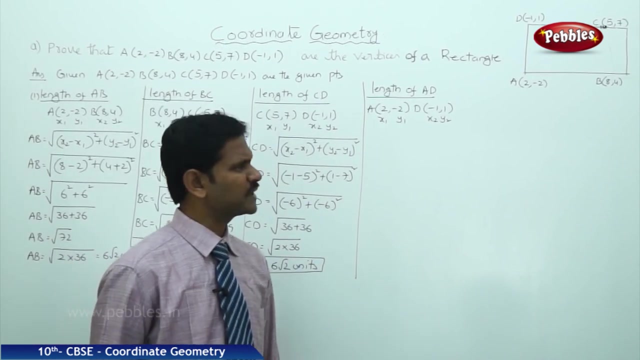 Now CD value is completed. Next length of AD: AD, That is, AD is A of 2 comma minus 2 and D of minus 1 comma 1.. Length of AD: A of 2 comma minus 2, D of minus 1 comma 1.. 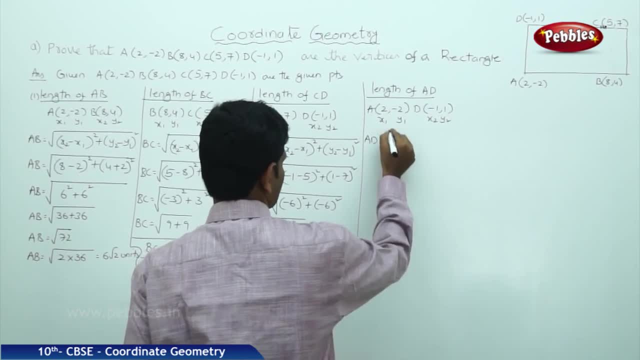 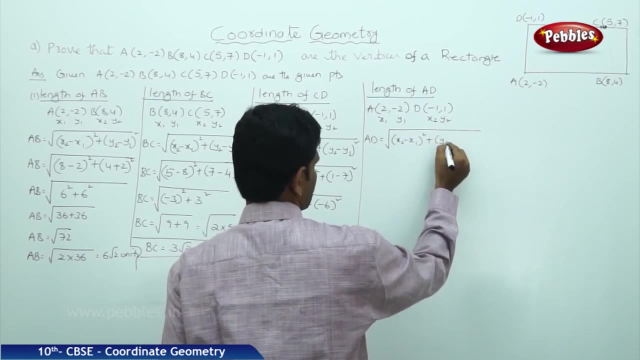 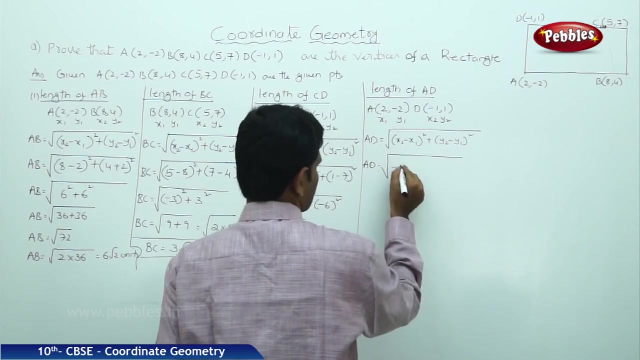 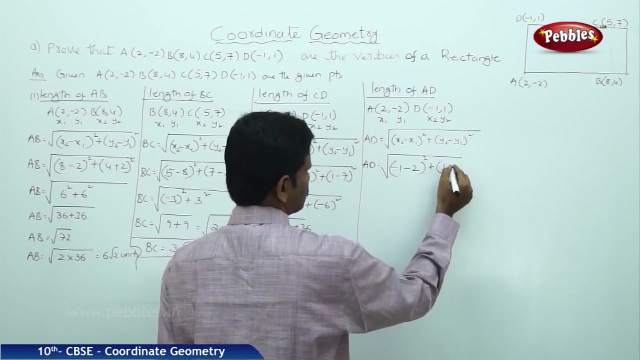 Now AD is equal to root over x2 minus x1, whole square, plus y2 minus y2.. AD is equal to root over x2 minus 1 minus x1 is 2 whole square y2 1, y1 is minus 2.. 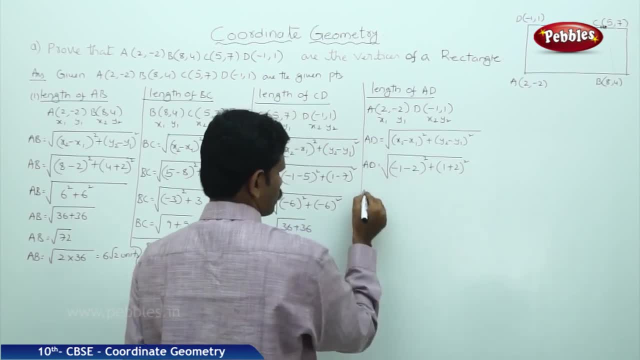 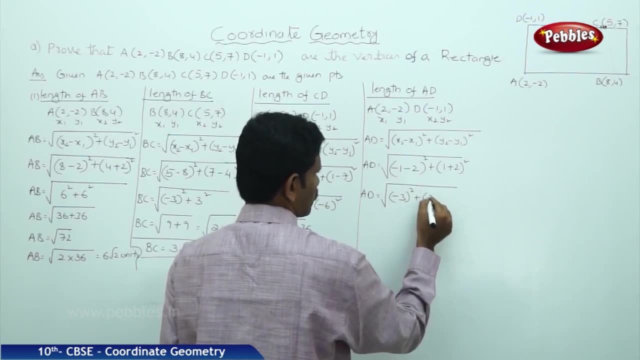 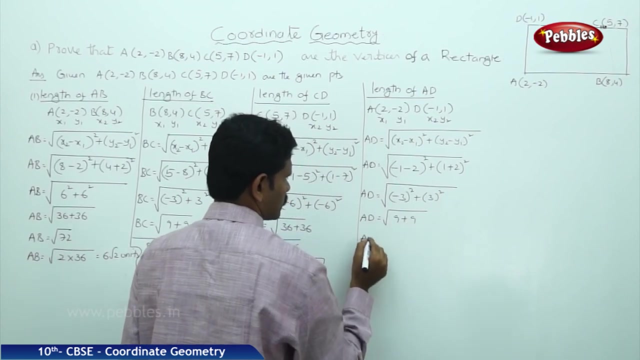 That is a minus into minus plus 2.. AD is equal to root over minus 3 whole square plus 3 square, AD is equal to root 9 plus 9.. Now AD is equal to 2 into 9.. 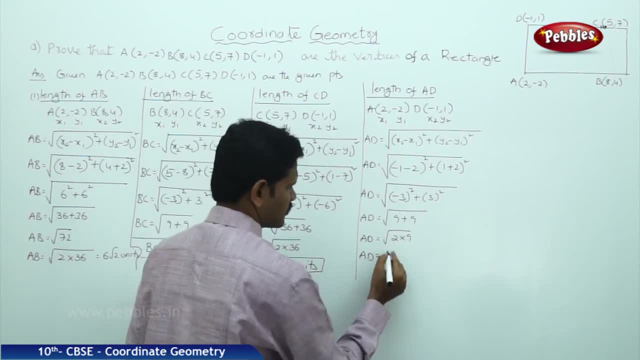 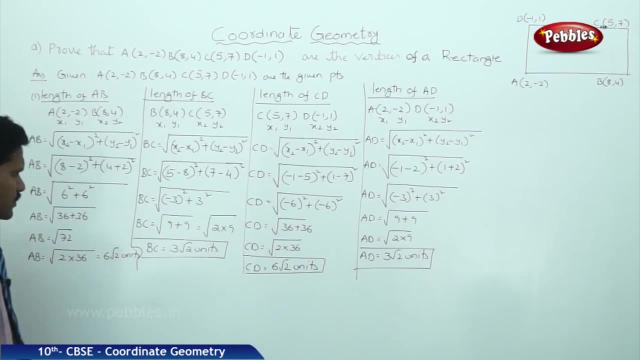 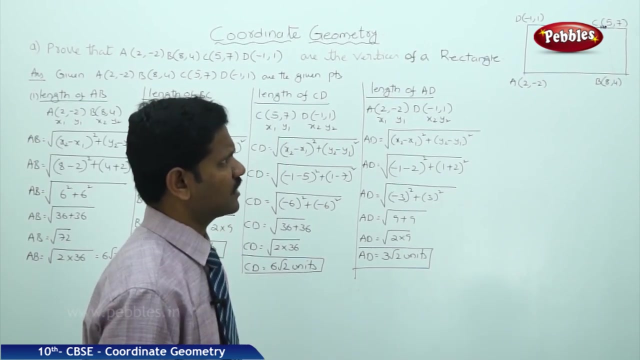 AD is equal to root 9 can be written as 3 root 2 units Now AB, BC, CD, DA, That is the length of 4 sides are completed. Then let us check opposite sides are equal or not. 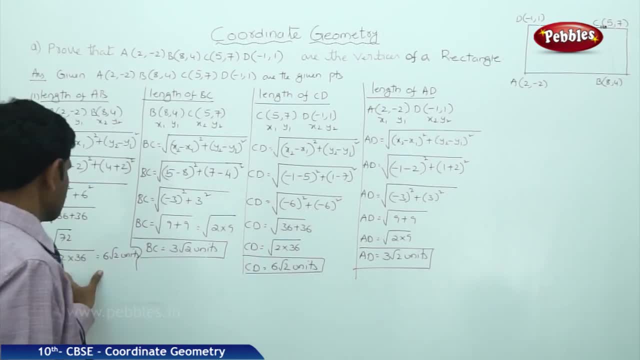 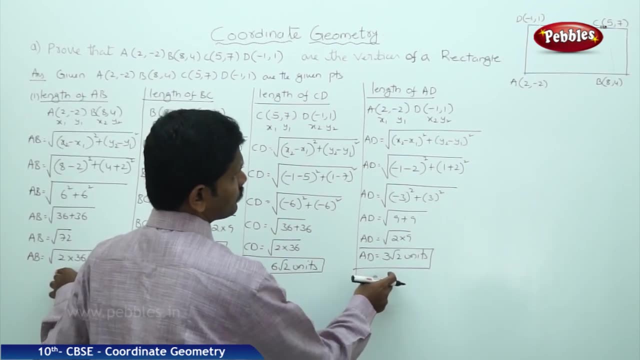 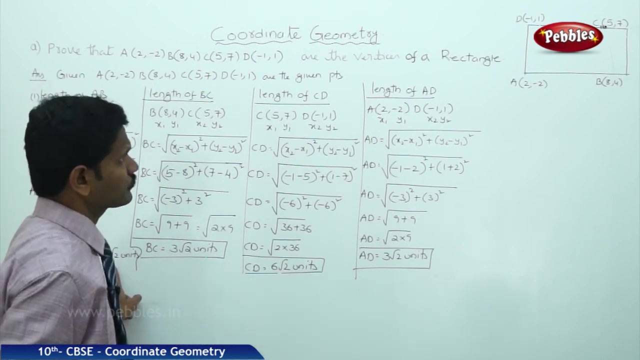 Value of AD is equal to root over x2 minus x2.. Value of AB: 6 root 2.. And value of CD. value of AB: opposite CD: 6 root 2.. Both are same. Next opposite side to AD is BC. 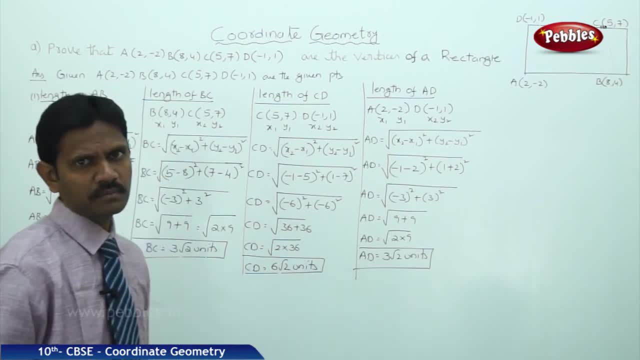 That is BC value and AD value. both are same. Okay, That means a quadrilateral in which two pairs of opposite sides are equal. Now, to conclude, this is: it is a rectangle. Now we have to do the verification of the diagonals. 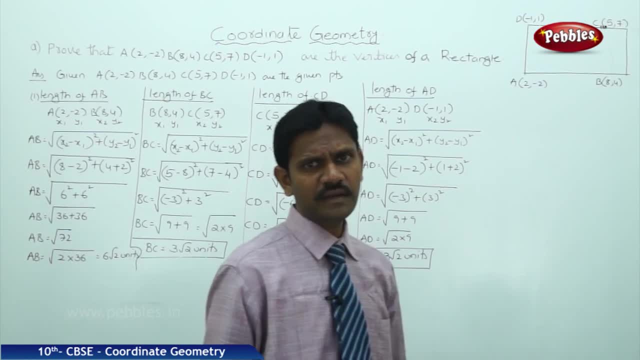 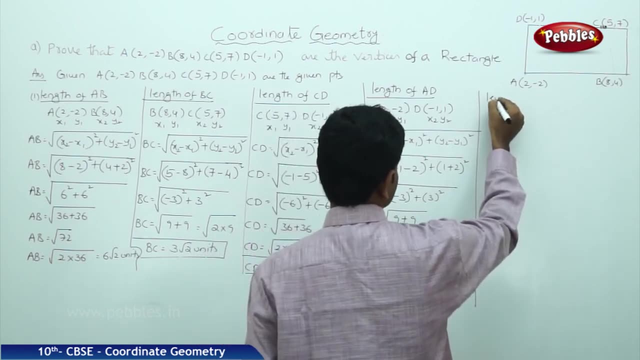 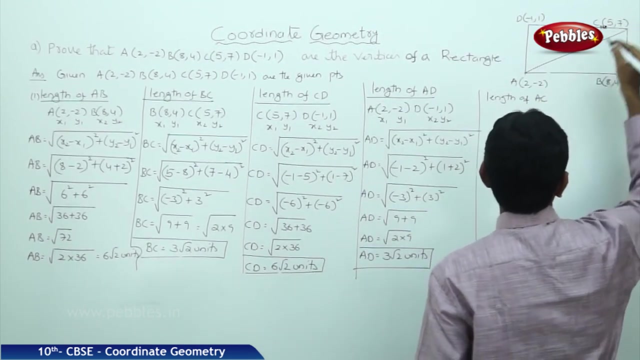 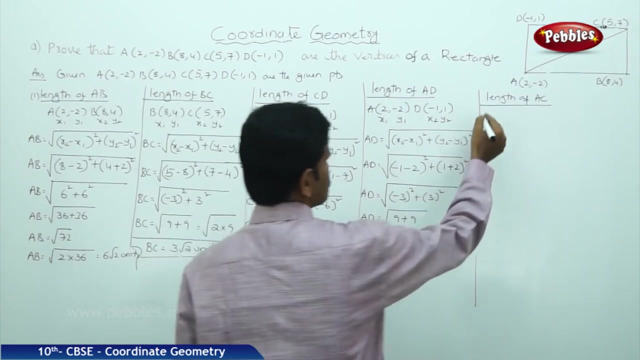 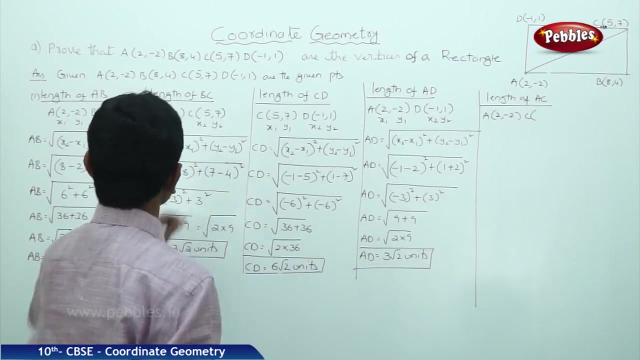 If diagonals are also equal, then it is called as a rectangle. Now let us follow Length of AC. Length of AC, That is A of 2 comma minus 2, C of C of 5 comma 7.. 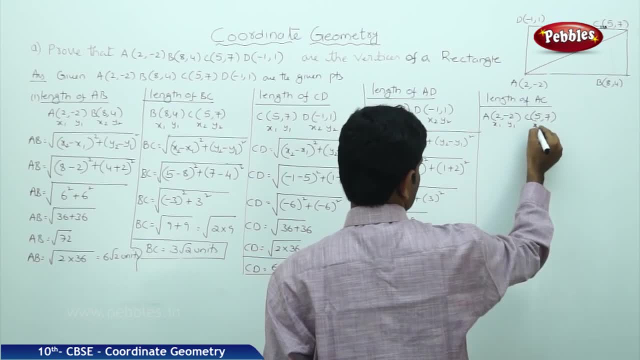 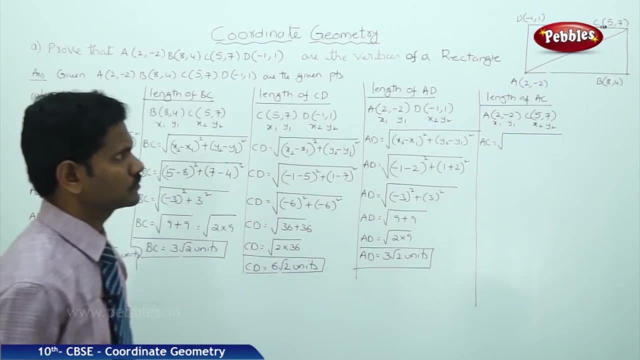 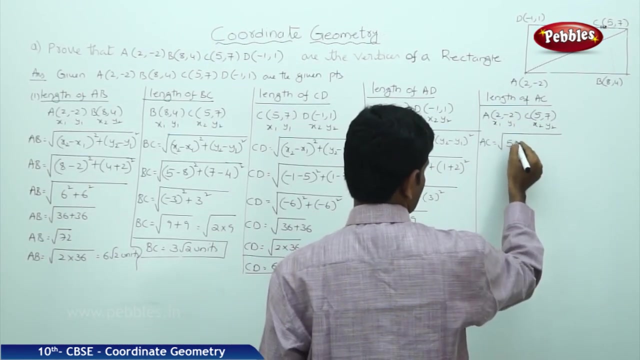 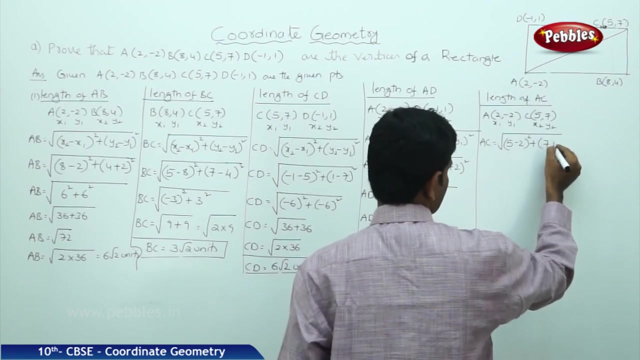 That is x1, y1, x2, y2.. AC is equal to root over. AC is equal to root over x2 minus x1, 5 minus 2 whole square plus y2 minus y1, 7 plus 2 whole square. 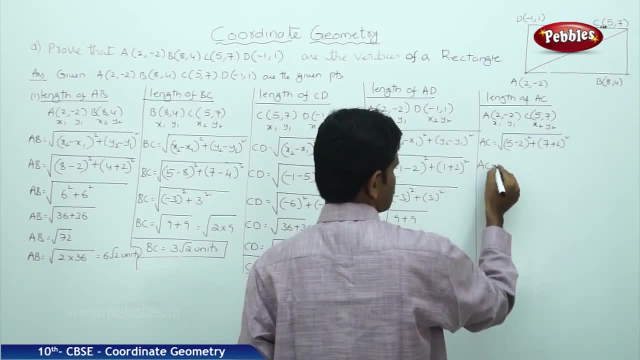 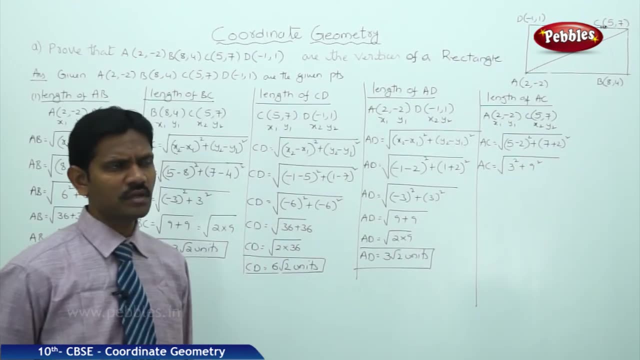 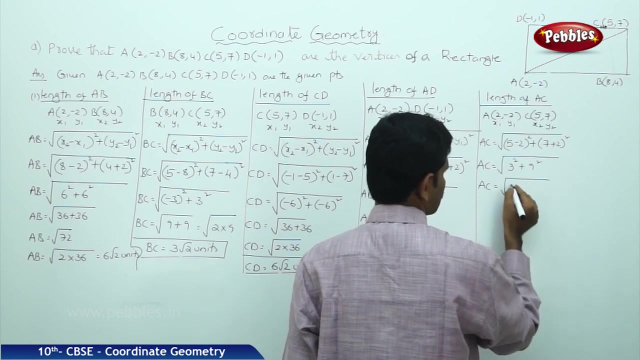 That is, AC is equal to root over 3 square plus 9 square, 5 minus 2,, 3, 7 plus 2, 9.. AC is equal to root over 9 plus 81.. 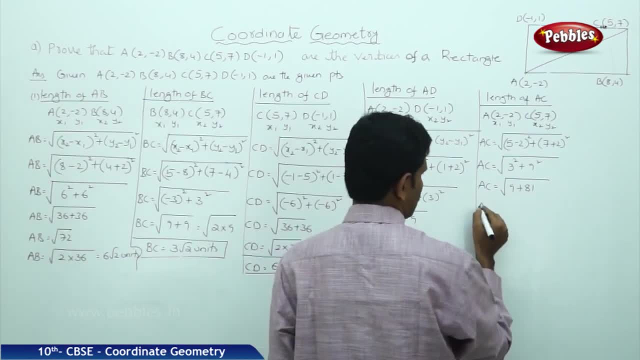 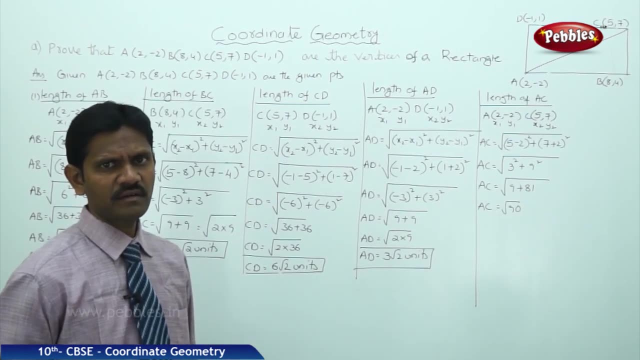 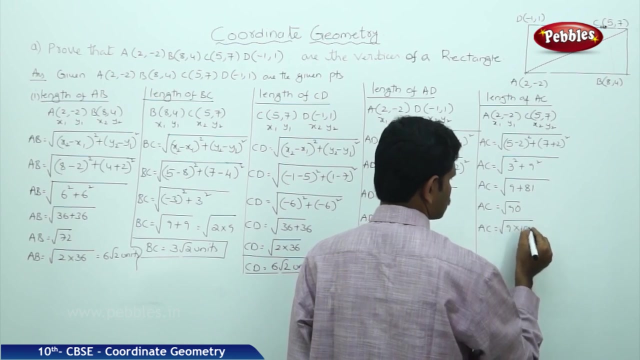 9 square is 81.. That is, AC is equal to root 90.. 81 plus 90.. Now AC is equal to, which will be break down into 9, into 10.. That is, AC is equal to. 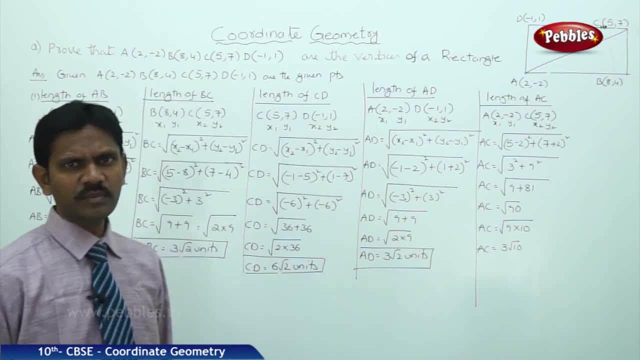 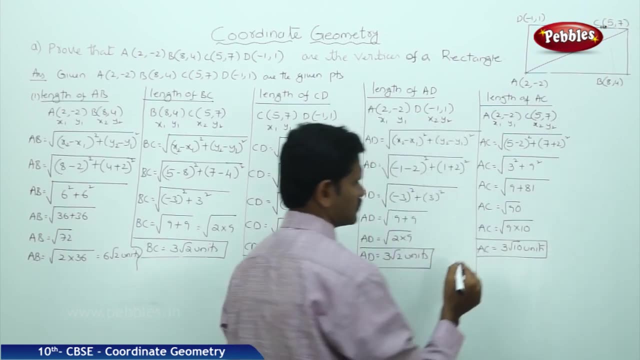 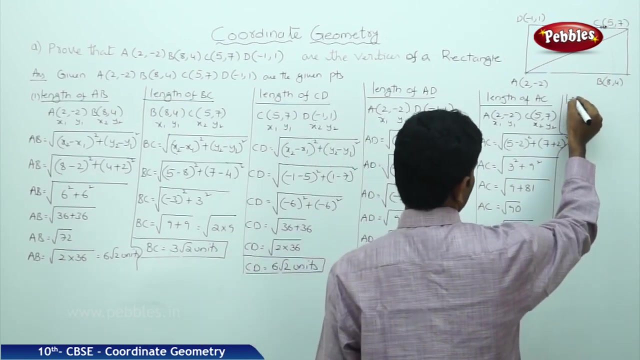 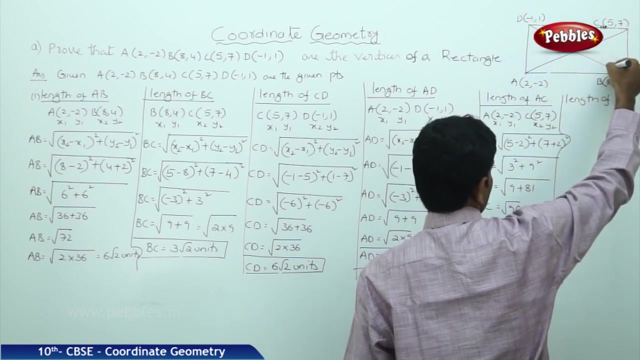 3 root 10.. Because root 9 can be written as a 3. Units, That is, AC value, is 3 root 10.. Now length of BC is our next step. Find the length of BD. 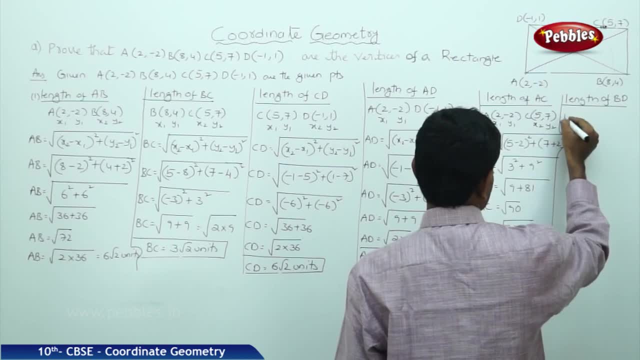 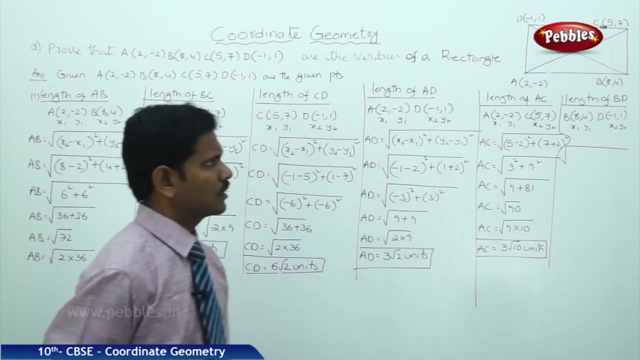 Now find the length of the BD, That is, B of 8 comma 4, D of minus 1 comma 1, x1, y1, x2, y2.. That is equal to root over x2 minus x1, whole square. 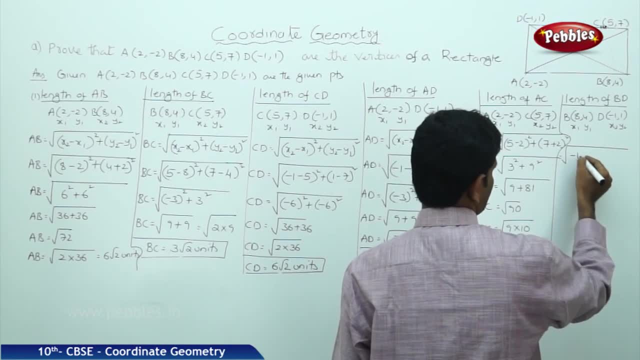 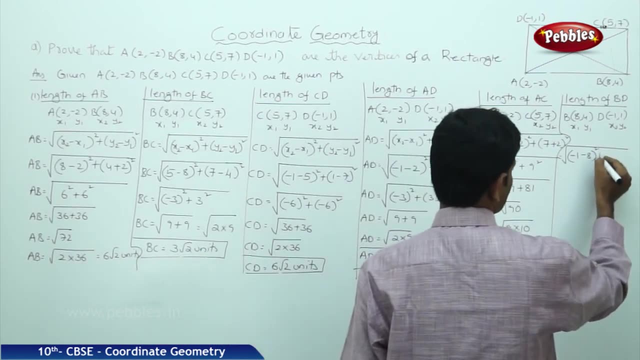 That is minus 1, minus 8 whole square Plus y2 minus y1 whole square. y2 minus y1 whole square. y2 minus y1 whole square. 1 minus 4 whole square, That is equal to. 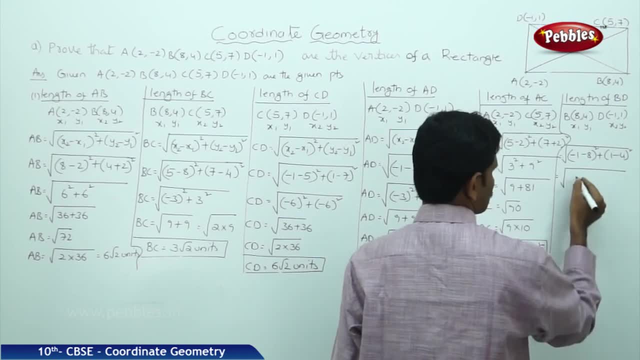 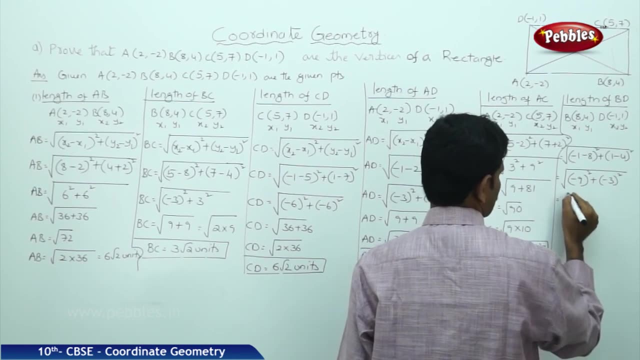 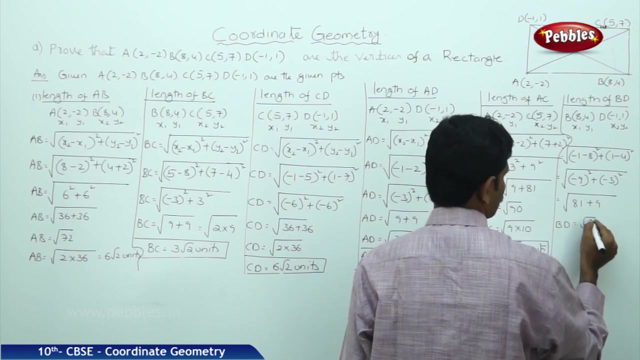 root over minus 9 whole square plus minus 3 whole square, That is equal to root over 81 plus 9.. That is, BD is equal to root 90.. BD is equal to root over 9 into 10.. 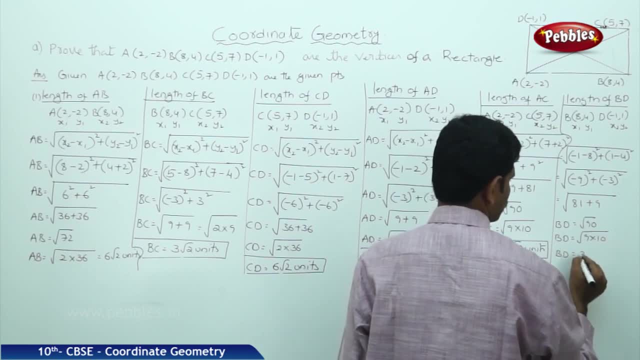 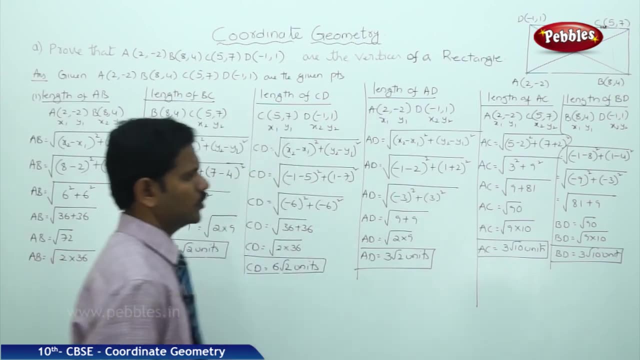 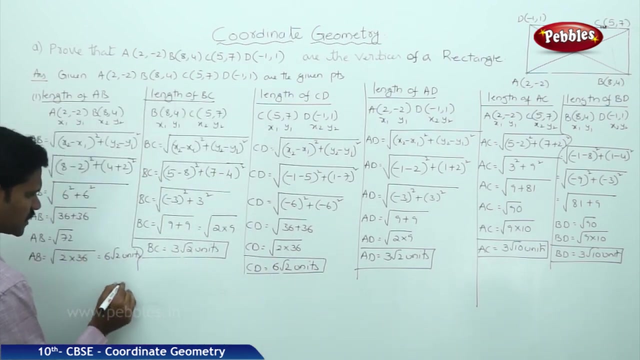 That is, BD is equal to. that is a BD is equal to 3 root, 10 units. Therefore, the diagonals are also equal. Therefore, we conclude that AB is equal to, BC is equal to, CD is equal to, AD is equal to. 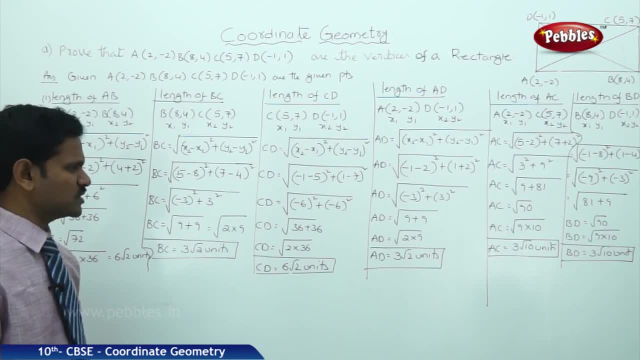 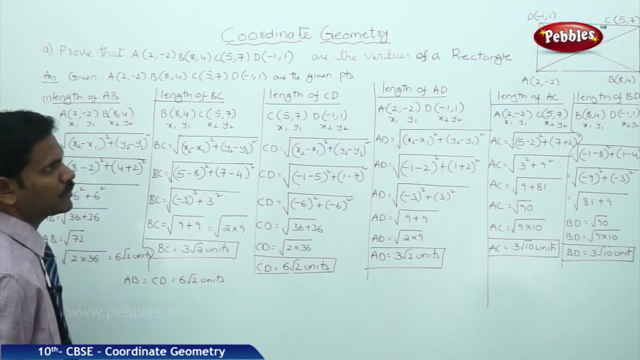 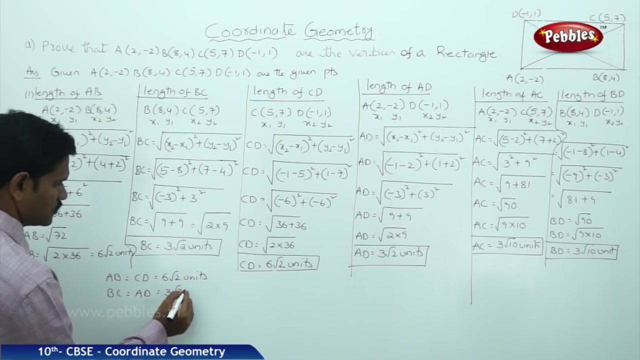 Therefore, from the given question, we conclude that the opposite sides, AB is equal to CD, is equal to 6 root 2 units, and one more pair, BC, is equal to AD, is equal to 3 root 2 units, and the diagonals: these two are the sides.